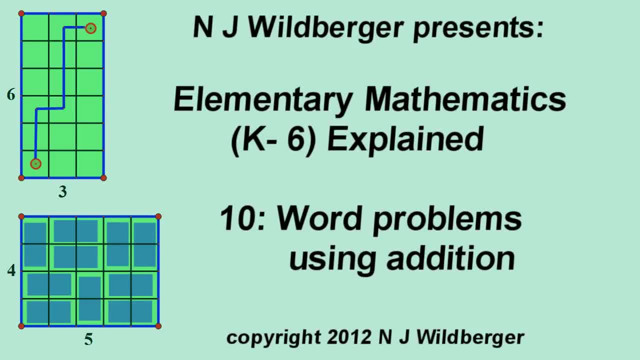 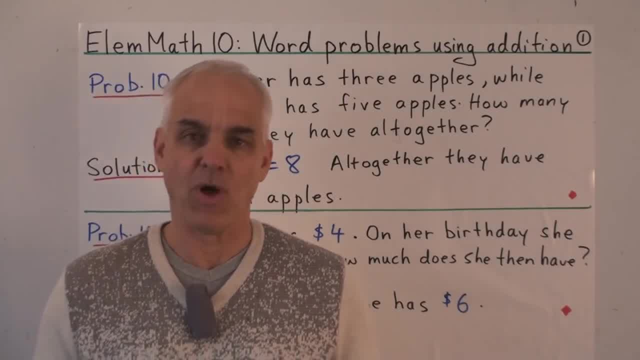 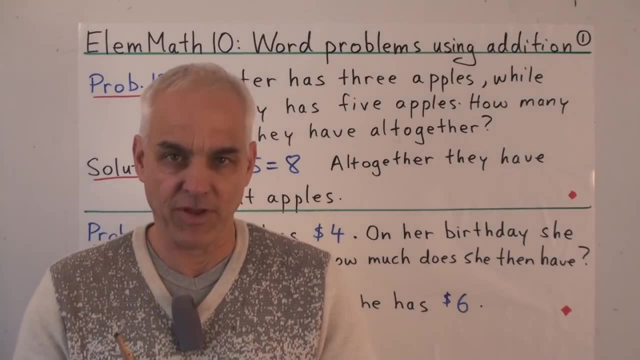 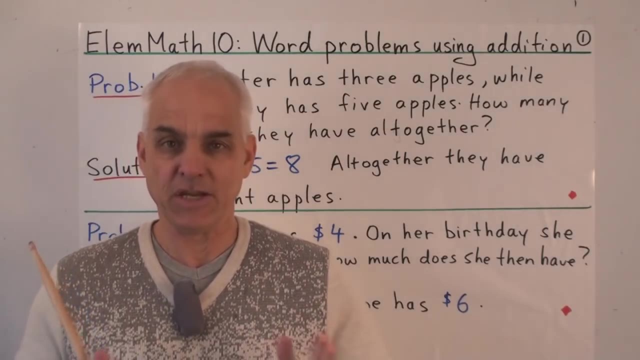 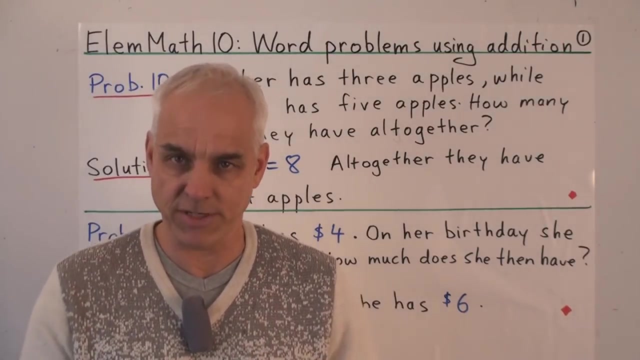 Welcome everyone, I'm Norman Wahlberger. In this video, we are going to introduce the idea of word problems in mathematics, And all the word problems that we are going to be considering are related to addition, Because that's pretty well the only operation that we're on top of at this point in this series on elementary mathematics, K-6.. 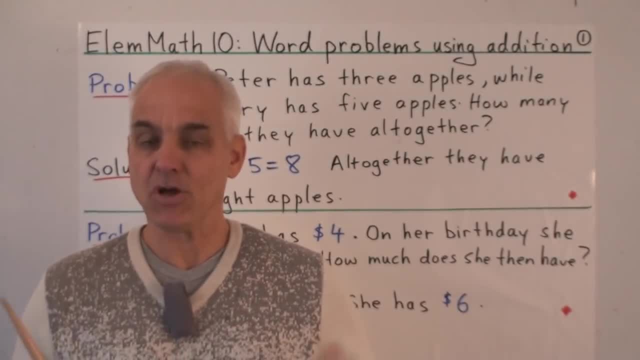 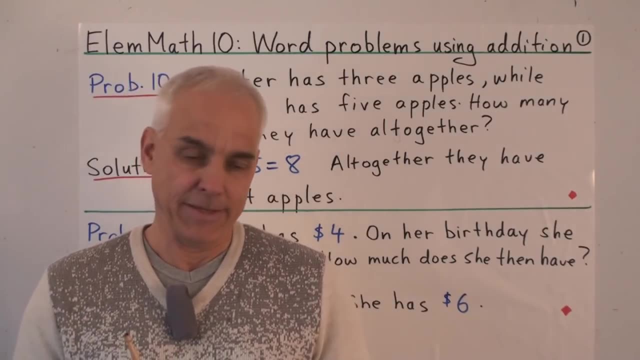 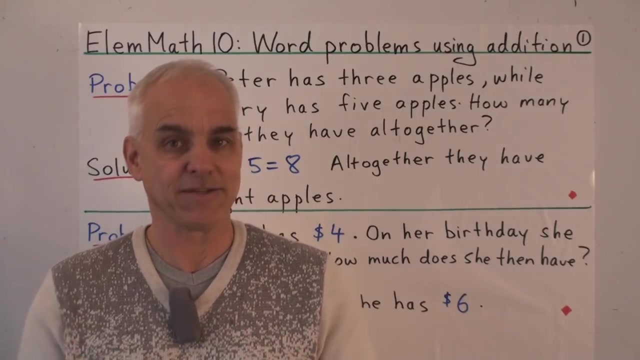 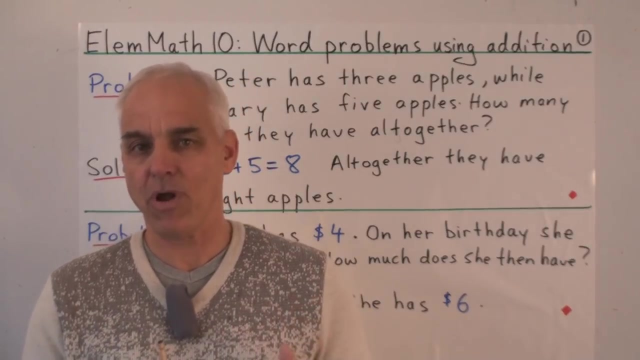 So we're going to practice some elementary additions in the context of sort of real life problems which are phrased in terms of sentences And, implicit at least, is the idea that the response should also be something of a sentence. So we're going to be looking at how to structure an answer to a word problem as much as how to get a solution for it. 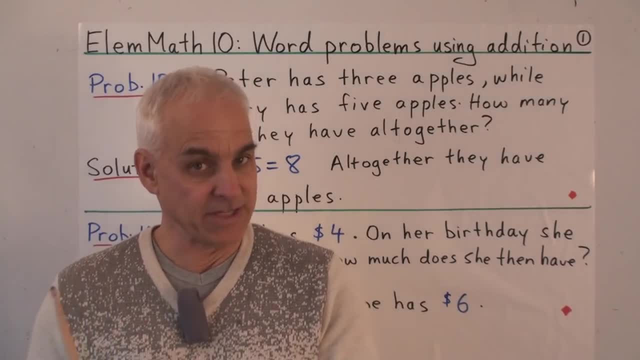 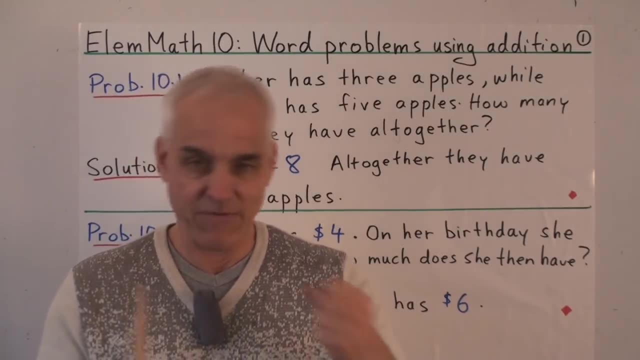 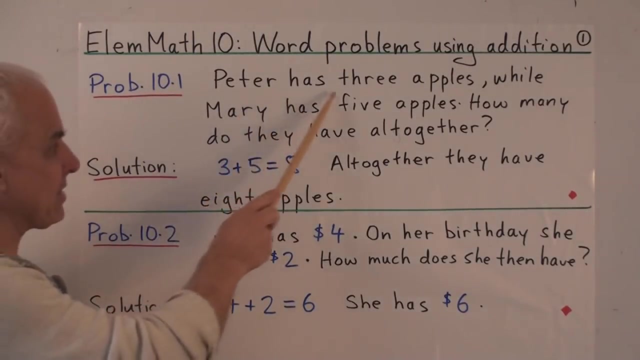 We'll be covering quite a range of problems, some very simple ones and then some not so simple ones, as we go a little bit further on into the lecture. So let's have a go. Our first problem is this one: Peter has three apples, while Mary has five apples. 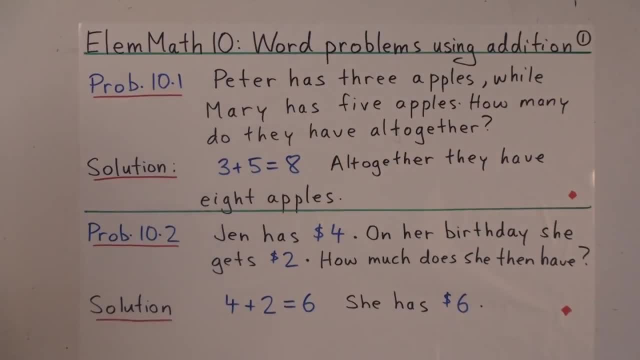 How many do they have all together? Well, the solution consists of identifying that the crucial quantities here are the three and the five. We have three apples and we have five apples, and the question is asking us to add them together, Because the question is asking: how many do they have all together? 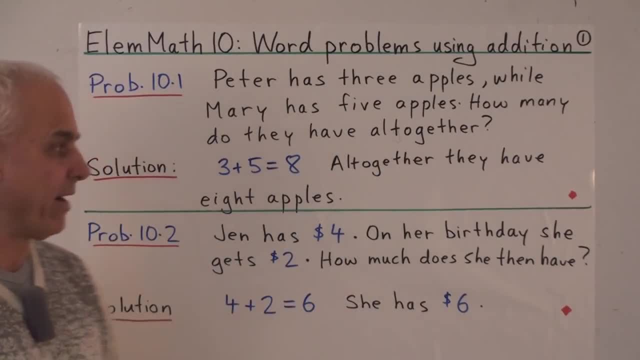 That's a kind of an adding. We're putting things in one big pile. So we have three and five and we're adding them together And hopefully we know by now that three plus five equals eight. Having done that computation, we can write the answer in a sentence form. 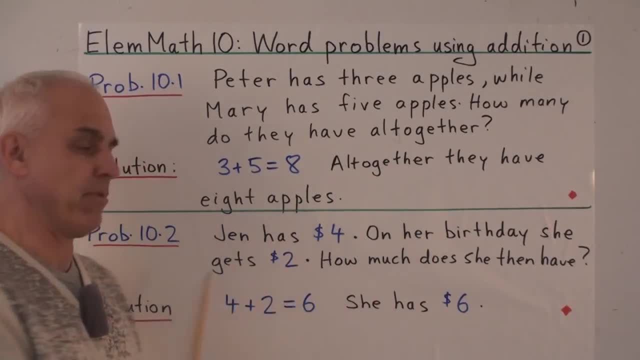 We can write: all together, they have eight apples. All right, our next problem: Jen has four dollars. This is the dollar sign, so that means four dollars. On her birthday she gets two dollars. How much does she then have? 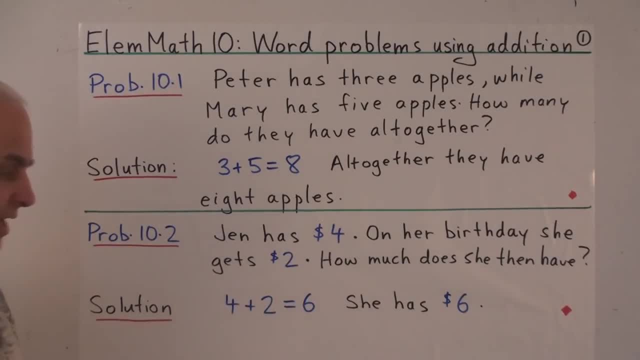 Well, it's a question of taking the four dollars and the two dollars and adding them together. She starts with the four dollars, She starts with the five dollars, She starts with the six dollars, She starts with the seven dollars, She starts with the eight dollars. 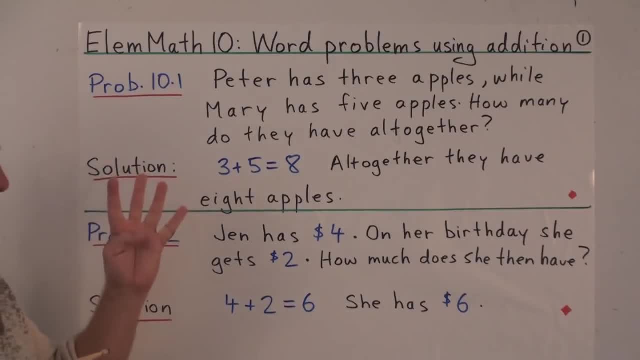 And then she adds two dollars to it, in the same way that we start with a rectangle with four here and then add two more there to get one with six. So there's the computation in terms of numbers and here's the answer: She has six dollars. 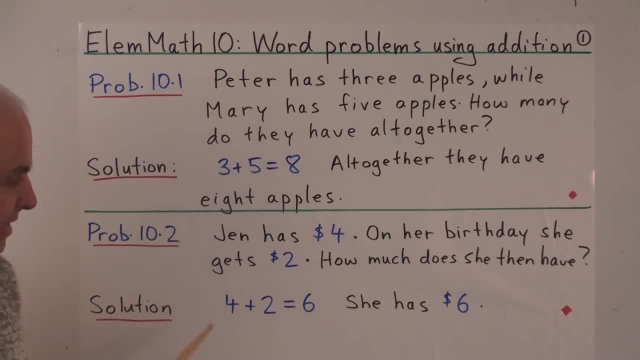 Notice that the equation that we write down doesn't have dollar signs in it. It's purely an equation involving numbers only. In the same way that this equation is an equation involving numbers only, this equation doesn't have any apples in it explicitly, It's only an equation having to do with numbers. 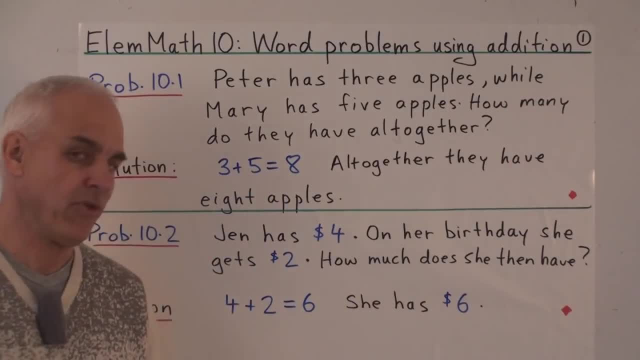 Whether this is three apples plus five apples equals eight apples, or whether it's three oranges plus five oranges equals eight oranges, or whether it's three dollars plus five dollars equals eight dollars. arithmetically, those three things are all the same. 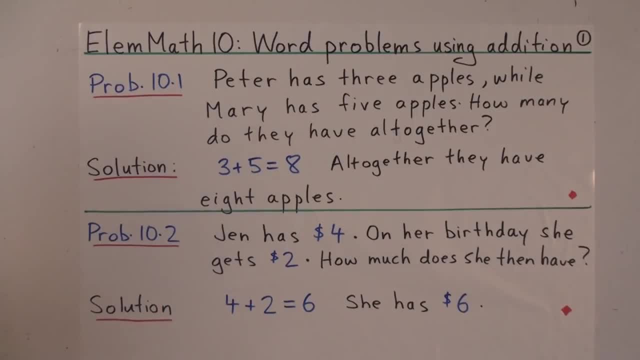 captured by this single equation, which doesn't have any units in it. Afterwards we can add the units Similarly here, once we've made the computation, we know that the answer is six. then the answer that we write down, we include the units. 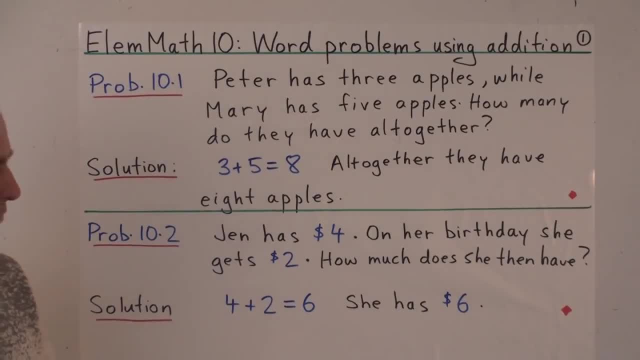 So we say she has six dollars, Referring back to the units that the question asked us about. So this question asked us about apples. We give an answer in apples. This question asked us about dollars. We give an answer. We give an answer involving dollars. 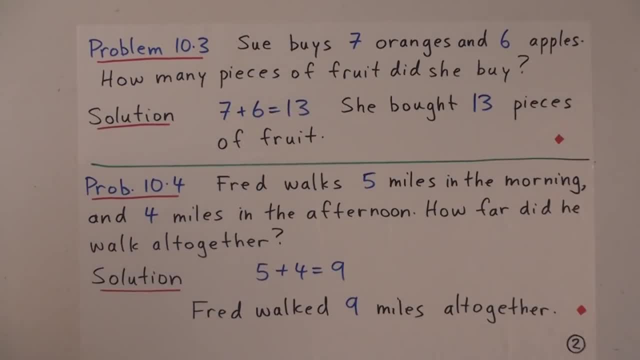 Our third problem has some fruit in it as well. Sue buys seven oranges and six apples. How many pieces of fruit did she buy? Well, you have to know that oranges and apples are both fruit, So the question is: including the oranges and the apples together? 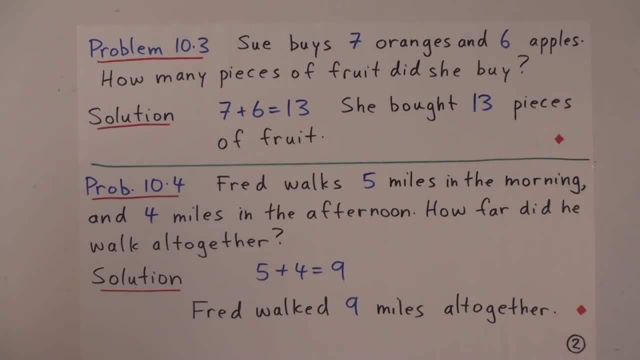 They're both fruit, So we still must calculate seven plus six, and hopefully we know that that's thirteen. But now we are talking about pieces of fruit rather than only oranges or only apples, So we might write down that she bought thirteen pieces of fruit. 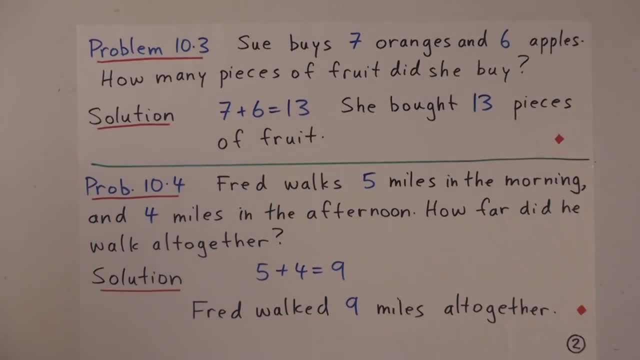 That would be an answer. Our fourth problem: Fred walks five miles in the morning and four miles in the afternoon. How far did he walk all together? Well, we have to add the number of miles he walked in the morning. We have to add that to the number of miles he walked in the afternoon. 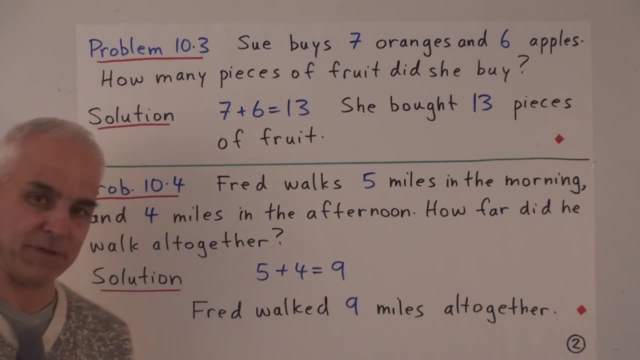 So it's five plus four. We have to figure out what five plus four is Now in this case. of course, it's easy, But if these were four, it would be a lot easier. But if these were four, it would be a lot easier. 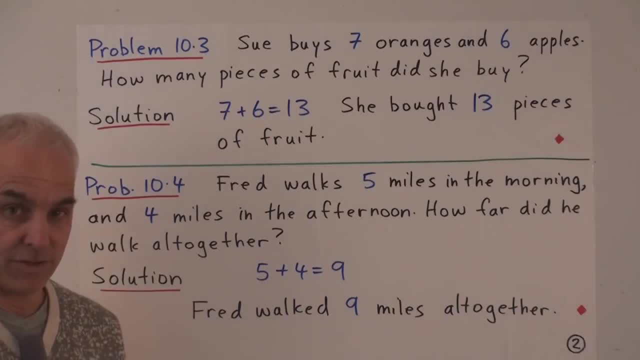 But if these were four it would be a lot easier. But if these were much bigger numbers it might involve a little bit of work to actually compute what that sum is. But we're just at the elementary stages here. So five plus four equals nine. 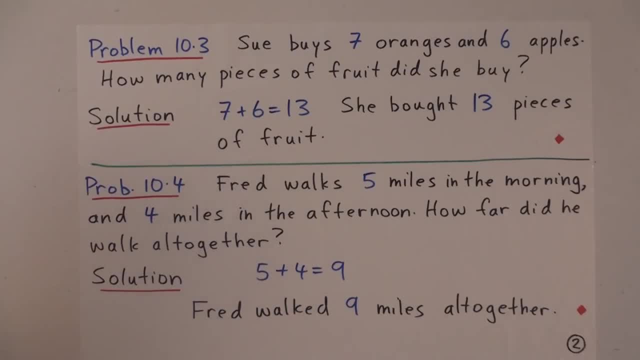 We can do that without too much problem. So there's the mathematical equation that captures the computation we're making And once we've made that computation, we can give the answer, Which is a sentence Which ends with a letter Which answers the question that we're given. 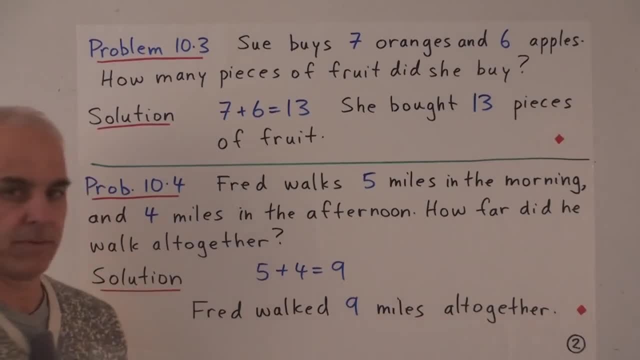 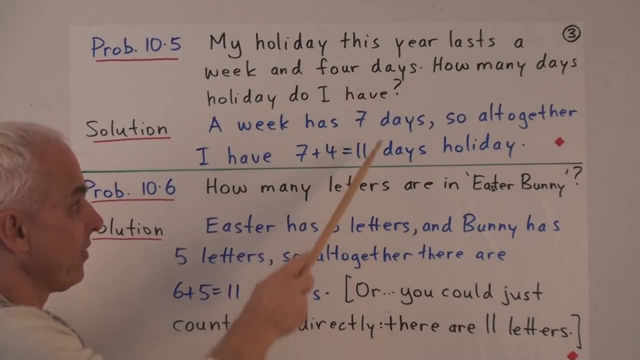 So Fred walked nine miles altogether. So our next problem is this one: My holiday this year lasts a week and four days. How many days holiday do I have? Well, we need to add the number of days in a week and the number four together for the total number of days. 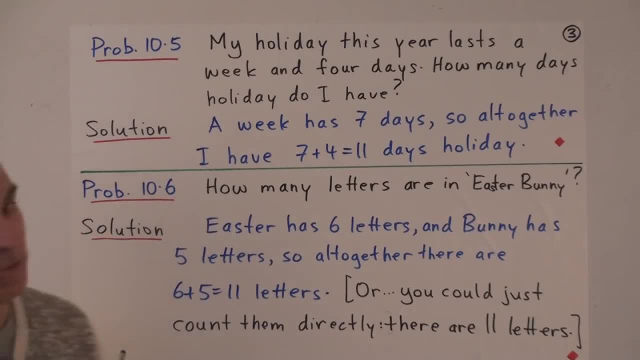 So it's an addition question. There's a little bit of possible ambiguity in the sense of: well, what do we mean by a week here? The standard interpretation is a week has seven days, But if you're thinking of a working week, then maybe you might only think of a five-day week. 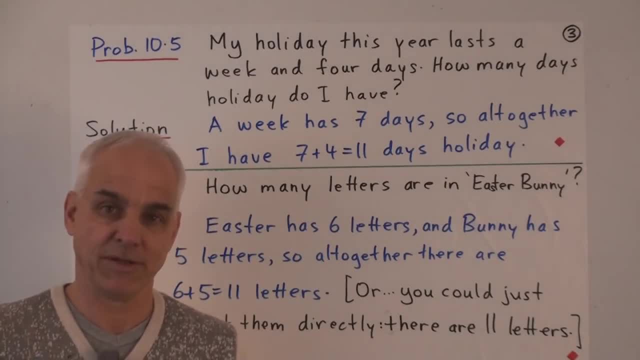 So sometimes it's necessary for us to interpret some ambiguity that may be in a question, Or maybe that we think is in a question, Perhaps because we don't understand something quite as well as we like. In this case, I'm going to resolve this by deciding for myself what the week means. 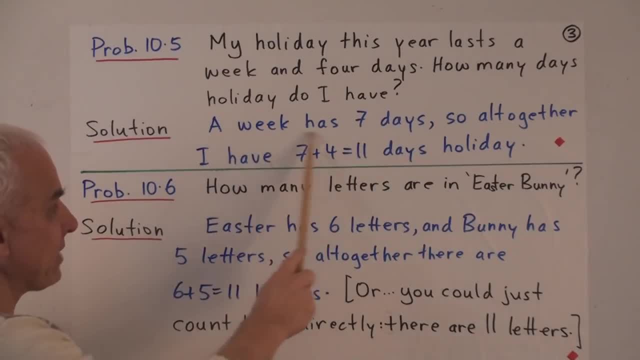 So I'm going to say a week has seven days And I'm going to write that down explicitly so that someone reading my solution can follow my train of thought. You might not agree with me that a week has seven days. You might think: well, we're talking about a working week with five days. 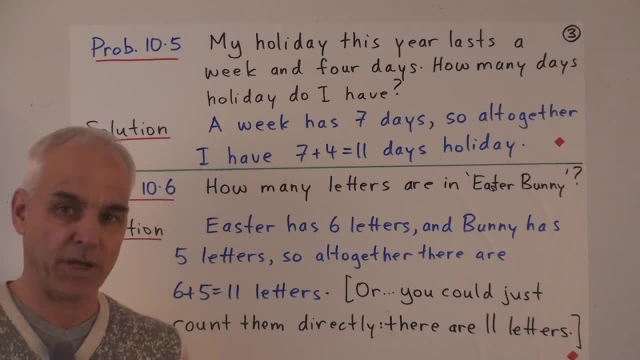 So when you read this you can clearly see that I'm at least working under the hypothesis that a week has seven days, So a week has seven days. So altogether I have seven plus four equals eleven days holiday. So I'm taking the seven days for the week and I'm adding the four extra days. 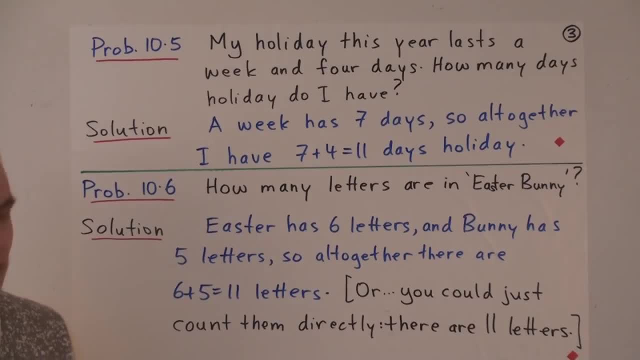 And then I have to make this calculation: Seven plus four equals eleven, And I'm going to put that equation inside the sentence. That is allowable in mathematics. Okay, when we're doing mathematics or writing mathematics, we often have equations as part of our structure. 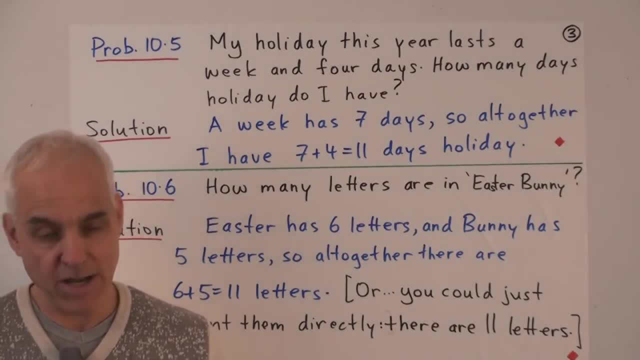 So your English teacher might not entirely approve, but still, in mathematics that's okay, And we will allow ourselves this insertion of an equation into a sentence. So note that I'm trying to explain what I'm doing so that someone reading it can follow my line of thinking. How many letters are in Easter, Bunny? Well, I'm going to do it this way. I'm going to say: well, Easter has six letters: One, two, three, four, five, six And Bunny: one, two, three, four, five. 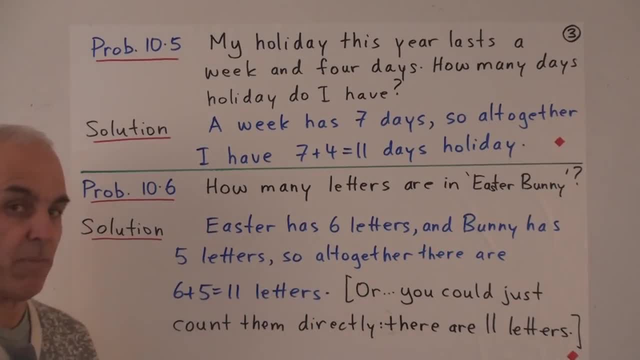 Bunny has five letters. So altogether I need to combine six and five. So altogether there are six plus five equals eleven letters. So again note that I've inserted this equation as part of my sentence structure. So altogether there are six plus five equals eleven letters. 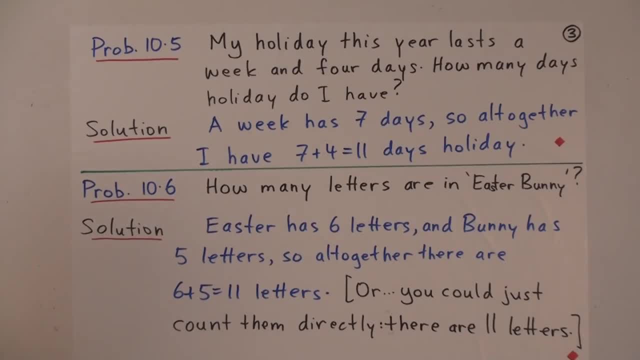 In this case, another possible solution would be to simply have counted them. to begin with, You could just count them directly and say: there are eleven letters: One, two, three, four, five, six, seven, eight, nine, ten, eleven. 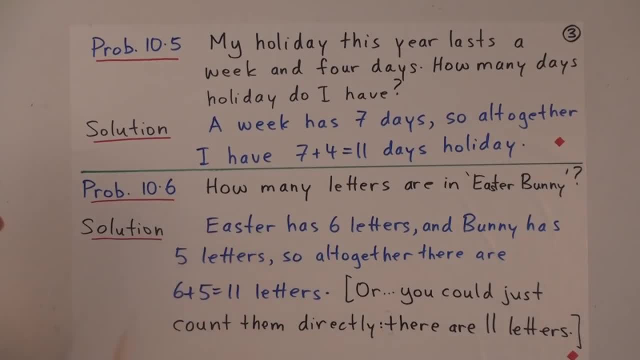 But in this case maybe it's a little bit more natural to look at the Easter, count those, look at the bunny, count those and then add those up. So I hope you're getting the hang of how one might write some mathematical solutions in words. 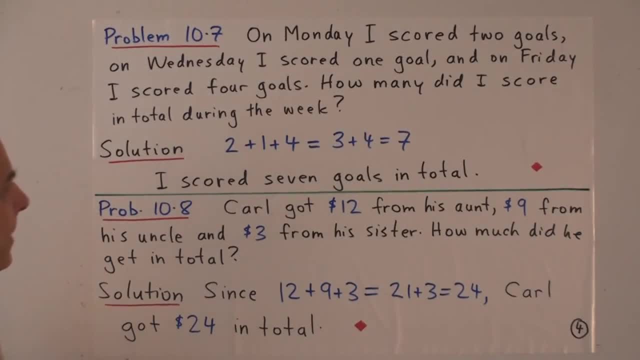 Let's have a few more examples. Problem number seven: On Monday I scored two goals, On Wednesday I scored one goal, And on Friday I scored four goals. How many did I score in total during the week? So I have to look through. 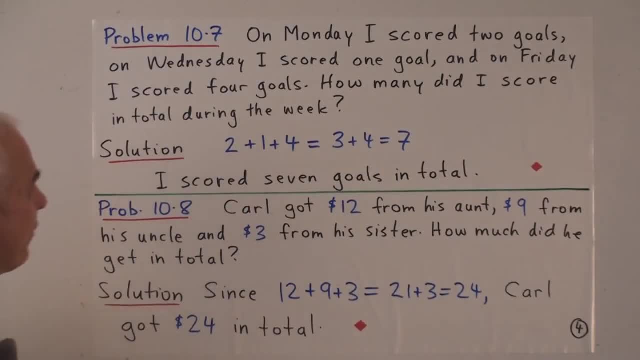 So on Monday I scored two goals- Okay, two is going to be important. On Wednesday I scored one goal. That one is going to be important. And on Friday I scored four goals. That four is important. So I'm going to add two plus one plus four. 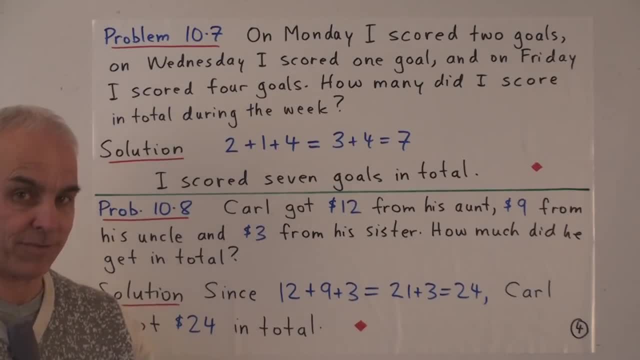 Now I'm adding three things together And I can combine this in a number of ways. I'm going to do the obvious and combine or add the first two numbers first. So the two plus one makes three. So in the second step I'm going to write three plus four. 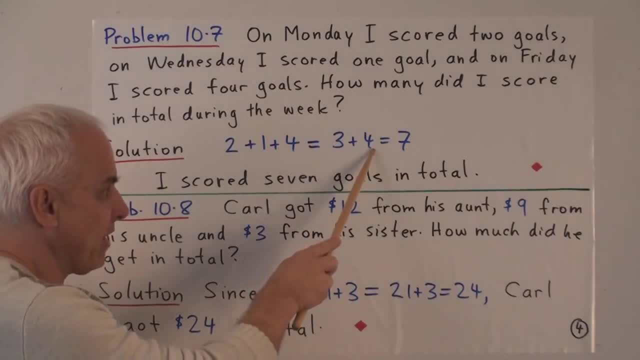 And then the last step. I'm going to combine three and four, Add those together to get seven. Having made the computation, I'm going to write down the answer with words, And I'm going to use words for the numbers, because the question that we were asked had the numbers in words as well. 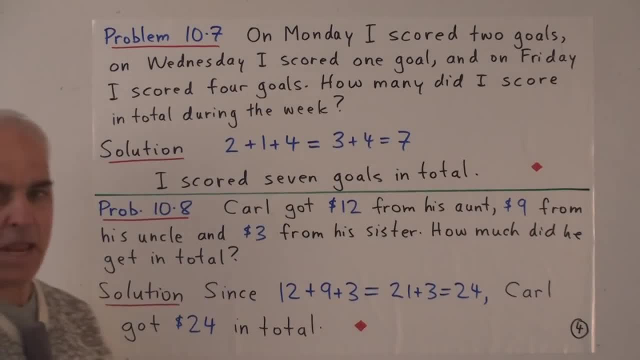 So I'm sort of going to reply in the same format, or a similar format to the way the question was worded to me. I'll say I scored seven, Seven goals in total. Problem number eight: Carl got twelve dollars from his aunt, nine dollars from his uncle and three dollars from his sister. 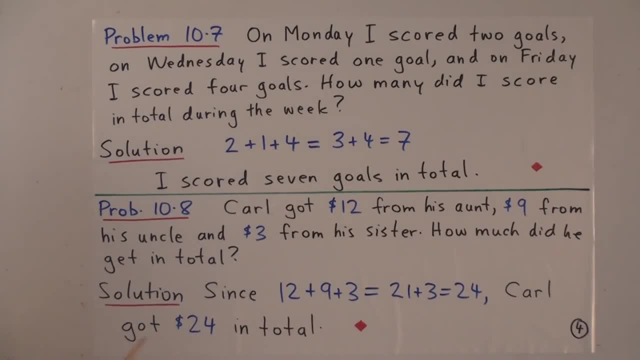 How much did he get in total? Well, we have to add those three different numbers: The twelve, the nine and the three. So twelve plus nine plus three. We can combine that in either of two ways. We can combine the twelve and the nine together, or the nine and the three together. 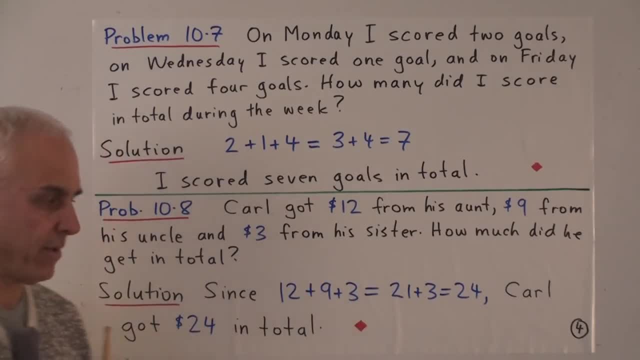 Let's combine the twelve and the nine together, That makes twenty-one, And then three more makes twenty-four, And I'm going to put that all in a sentence. So since this equals twenty-four, Carl got twenty-four dollars in total. The actual equation that I wrote down doesn't involve dollar signs directly. 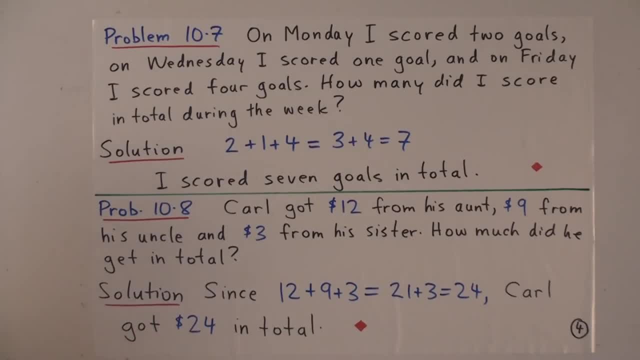 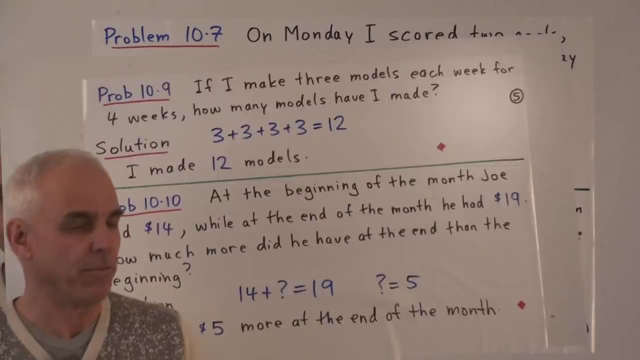 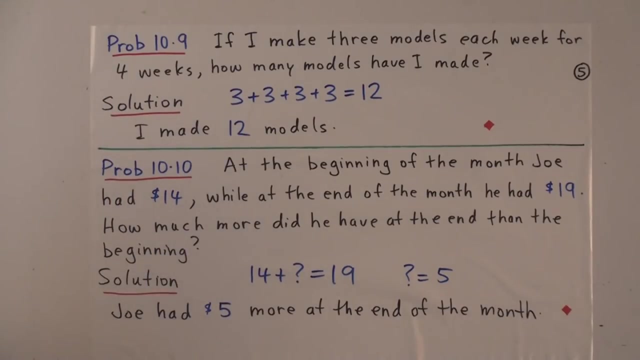 I introduce the dollar in the final answer- Twenty-four dollars in total- making sure that the units that I'm talking about correspond to the kinds of units that the question was asking about. Our ninth problem: If I make three models each week for four weeks, how many models have I made? 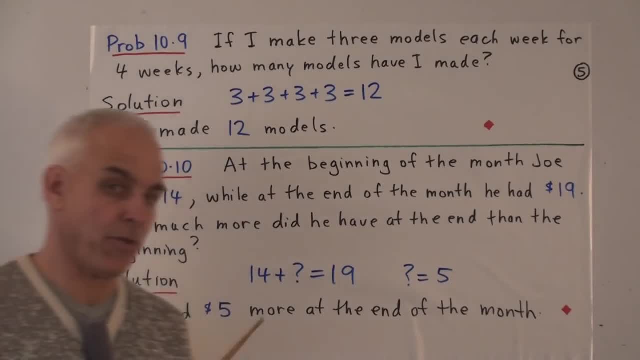 Now, later on we're going to learn that this is probably more naturally a multiplication question, But for now let's just use addition. So in the first week I make three models. In the next week, another three. In the third week, another three. 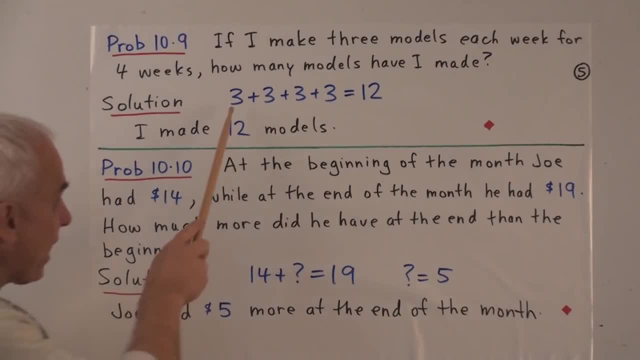 In the fourth week, another three. So I have to add three plus three plus three plus three. That three is for the first week, That's for the second week, That's for the third week, That's for the fourth week. And what is three plus three plus three plus three? 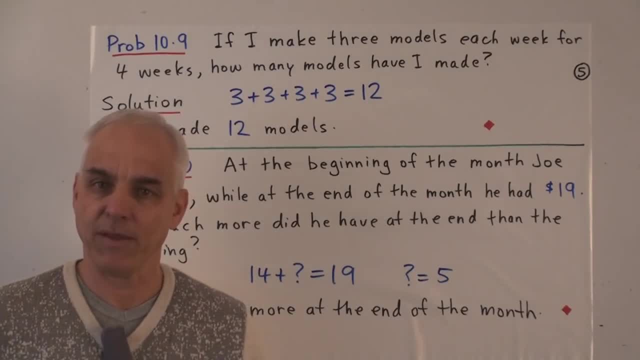 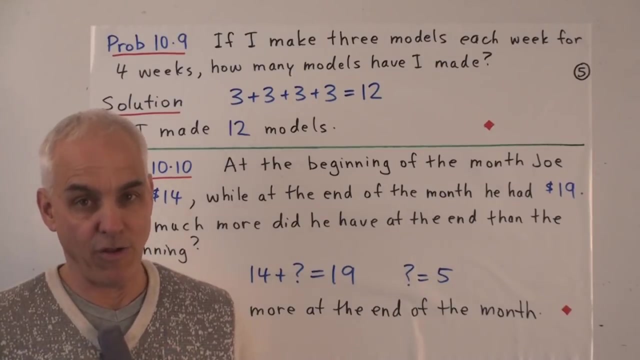 Well, that's a situation where we're talking about multiples of three. Every time we add three, we're going up in the chain of multiples of three, And I remind you that the multiples of three go three, six, nine, twelve, fifteen, eighteen and so on. 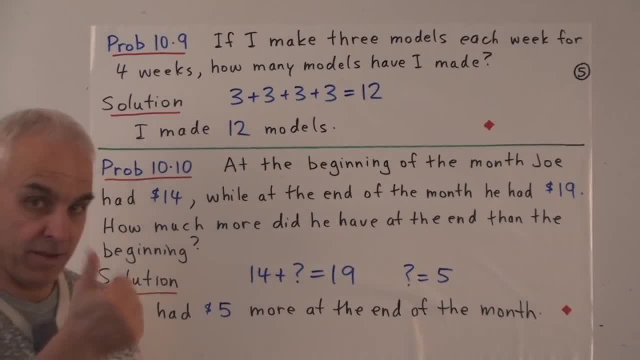 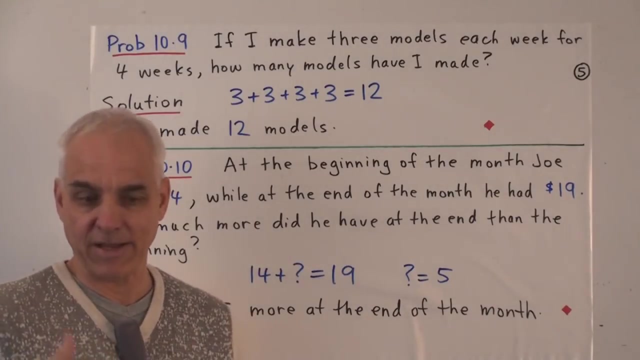 So the first: four, three, six, nine, twelve. So it's nice to have some experience with the multiples, To have gone through those beforehand, so it doesn't take you too long to go read up that ladder: Three, six, nine, twelve. 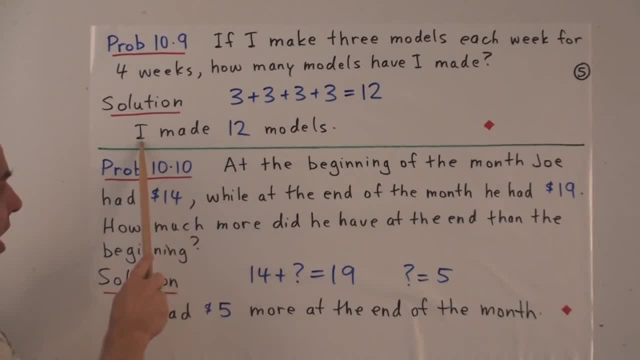 There are twelve altogether. So the answer: I made twelve models. Our tenth question, Our tenth problem: At the beginning of the month Joe had fourteen dollars, While at the end of the month he had nineteen dollars. How much more did he have at the end than the beginning? 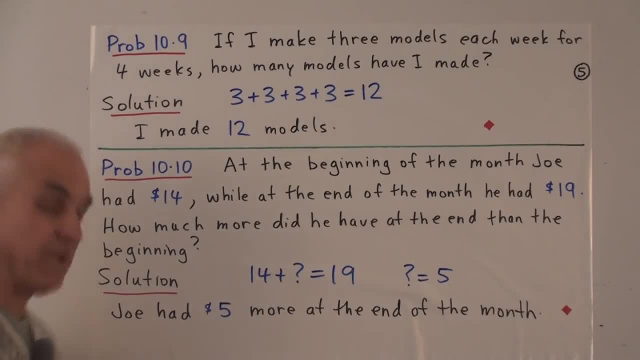 So we're starting with fourteen, We're adding some mystery amount And at the end we get nineteen, And we'd like to know what is that mystery number that we added to fourteen to get nineteen? Well, we can kind of do it by trial and error. 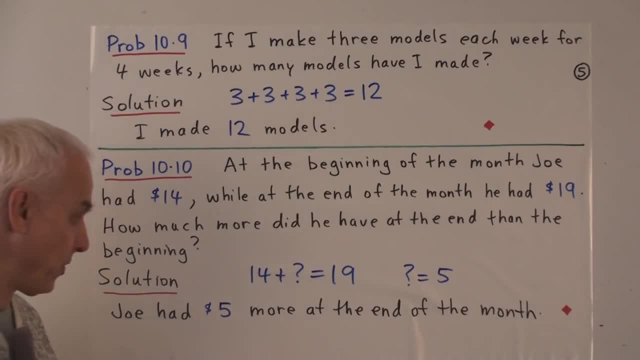 If we added one, then we would have gotten fifteen. If we had added two, we would have gotten sixteen. If we had added three, we would have gotten seventeen. Four would have given us eighteen. Five gives us nineteen, So the mystery number is five. 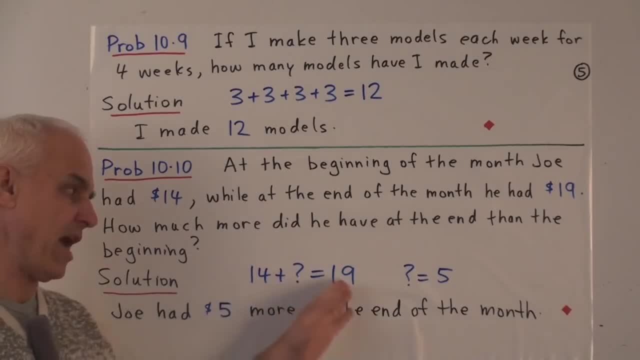 Or if you know your addition table, you know the four plus five equals nine, So that's got to be a five. And so then now, at the end, we answer the question in the same style as it's given to us. Joe had five dollars more at the end of the month. 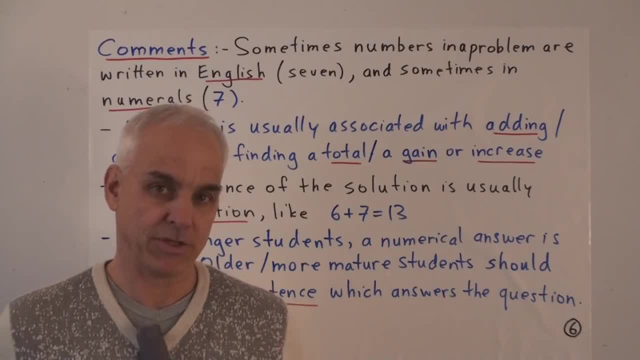 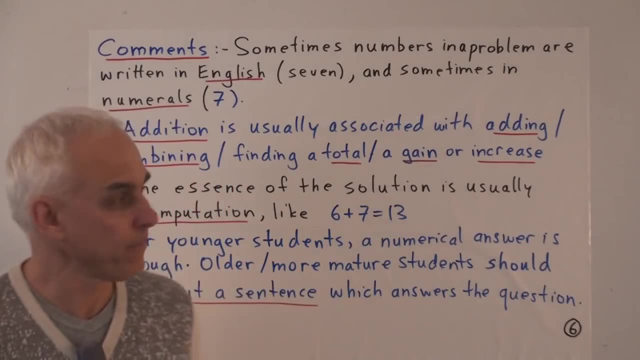 Here are some comments about the problems that we've been looking at, The kinds of things that can occur, The kinds of things to watch out for. The numbers that appear in a problem are sometimes written in English, like seven, this way, And sometimes they appear in numeral form like this: 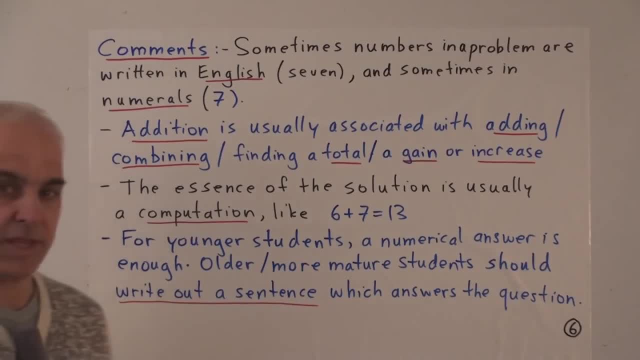 We've got to be able to work with either of them confidently, So we need to know, of course, how to convert the English names for the numbers to the numeral form. An addition problem is usually associated with adding or combining things, Or finding a total. 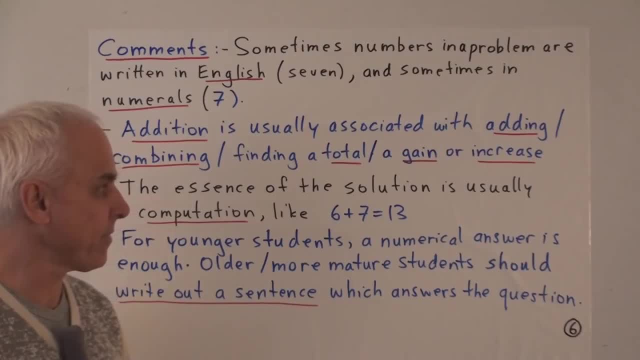 Bringing things together. It's often associated with a gain or an increase. These are all words or ideas that tend to make you think you have an addition problem going on here. The essence of the solution is usually contained in a computation or a calculation. 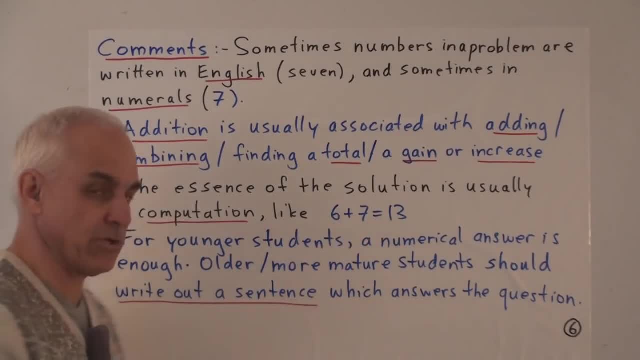 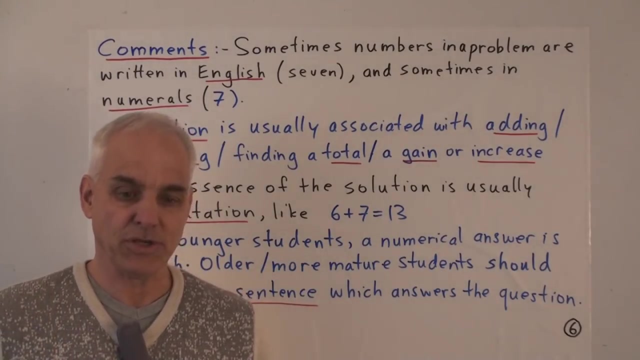 Like six plus seven equals thirteen, And it's quite reasonable to in your solution to actually write down that calculation explicitly. Now for younger students, a numerical answer is enough. If you're given a very young student, you ask him: Bob had three apples and then someone else gave him four apples. 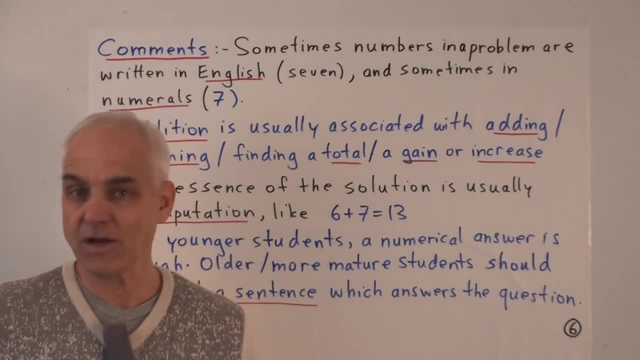 How many apples does he have altogether? The young student will just say Seven. That's probably all that they will say. If they write something down, they will only write down the number seven, And that's perfectly fine for a young student. 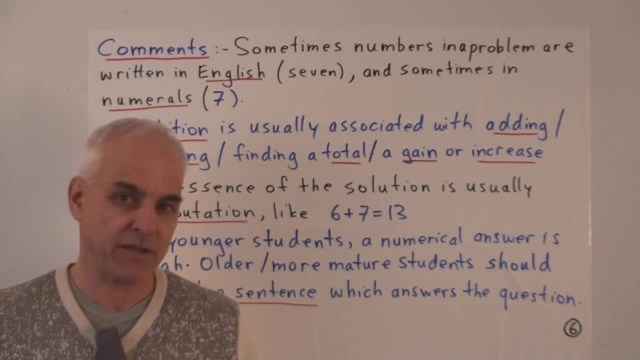 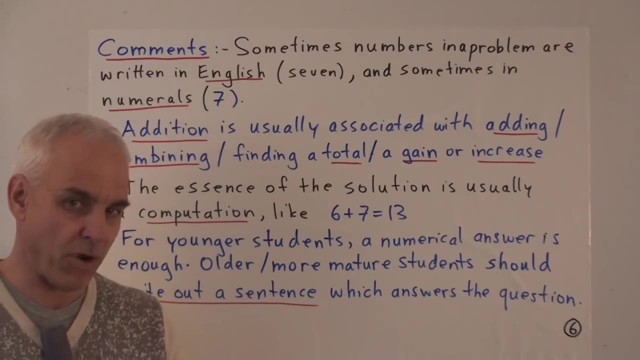 A little bit at a later stage. we can expect the student to write down the actual calculation. To write down: three plus four equals seven, That equation that represents or records what was going on in their mind. They made a calculation, They made a calculation and we can write down on the paper what calculation we actually made. 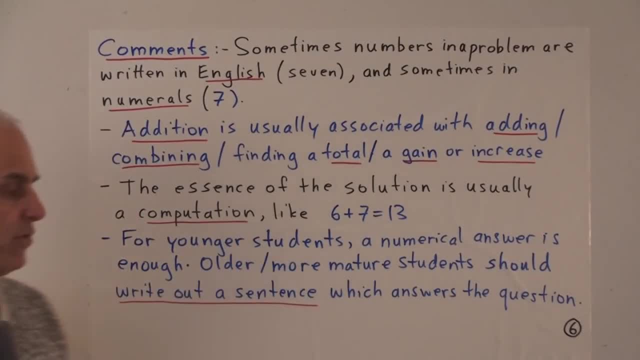 Now older or more mature students, which is probably most of you, should write out a sentence which answers the question. So you should aspire to writing out a solution which is an English sentence Which contains the information that someone requested of you. So, for example, you can imagine this question has been given to you by your boss. 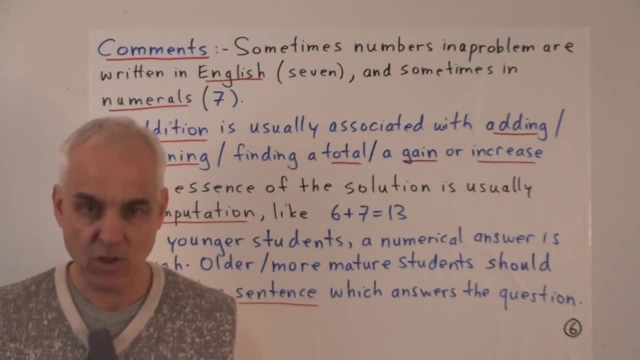 You're getting an email, You're getting a memo, There's a question. You want to respond to that Not just with a number, But in a sentence form, so that the person reading it can get a sense of what question this is answering. 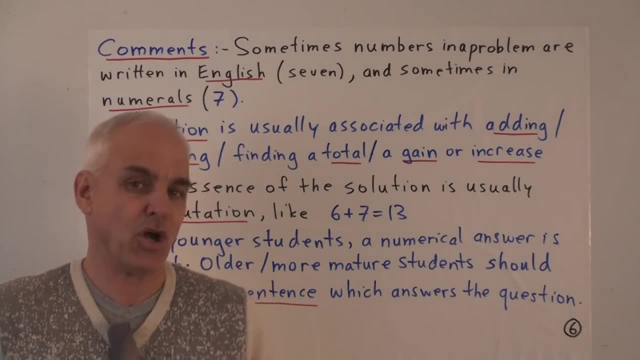 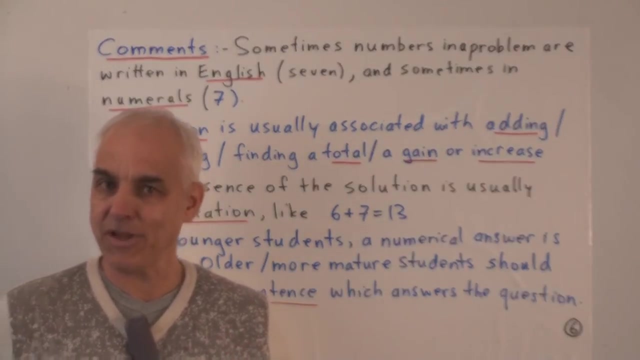 So you reflect part of the question back in the answer, Which makes it easier to recognize that this answer goes with this question. Where maybe this answer goes with this question, There's also the issue of the logical clarity of what we're doing In mathematics. we want to explain ourselves. 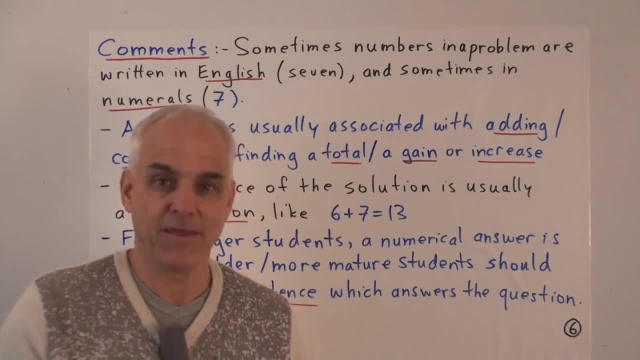 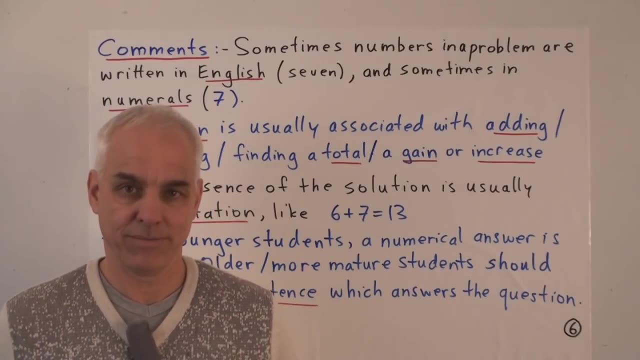 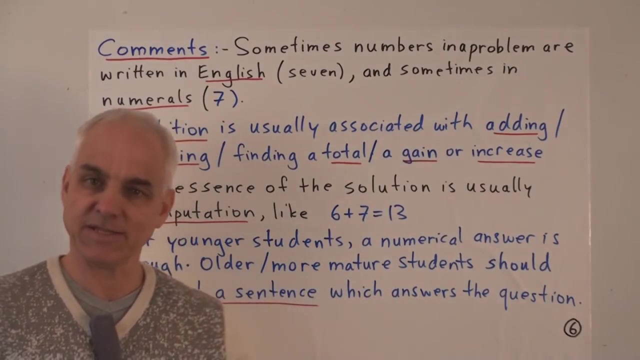 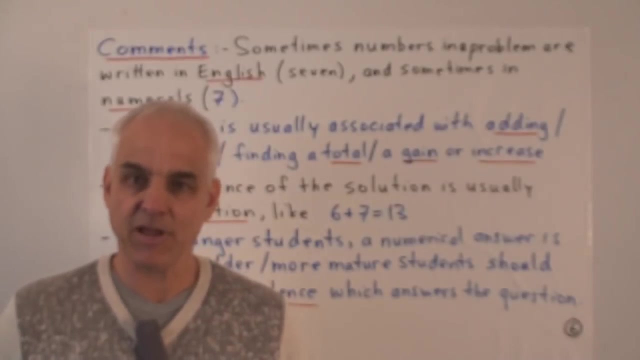 We want to convey in a simple, concise way What it is that we're doing. We want to have a record of our thoughts, And these word problems are moving us in that direction: The idea of expressing ourselves logically, Putting down what is necessary. 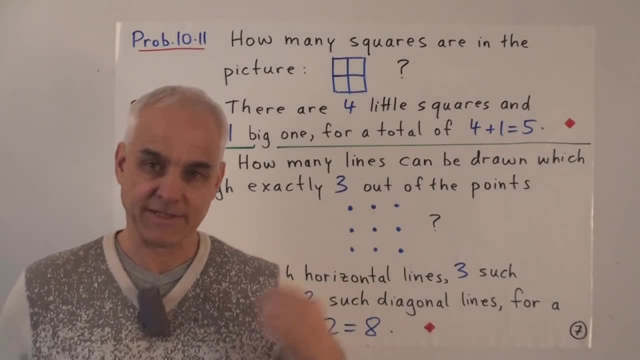 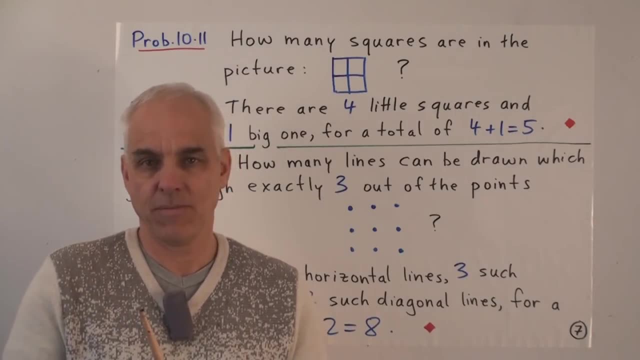 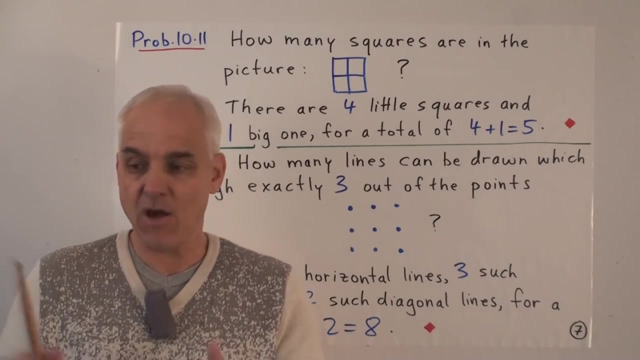 But not much more than that. Here are a couple of somewhat more sophisticated problems That show us that addition and counting are often very closely connected, So a lot of counting questions where you're asked to find how many of such and such there are. 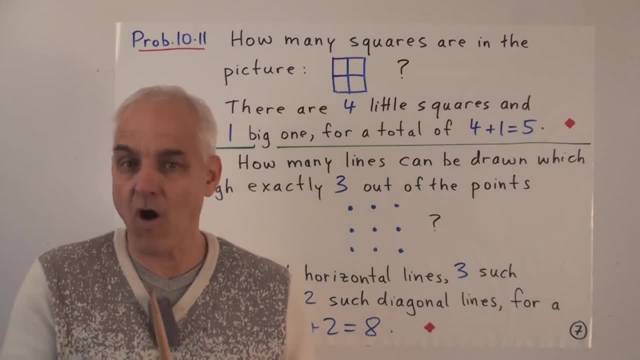 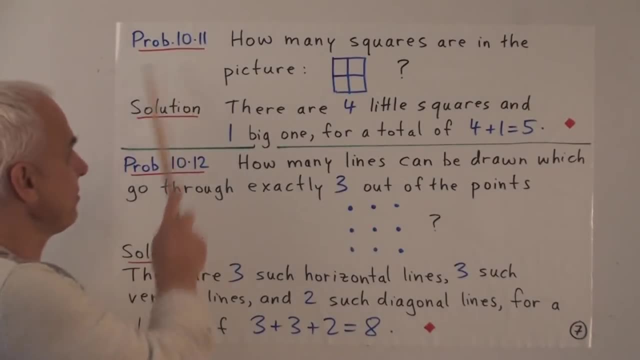 Are really, in some sense, addition questions, Or at least they involve some addition as part of solving the problem. Have a look at this question: How many squares are in this picture right here? Well, there's one square, There's another one. 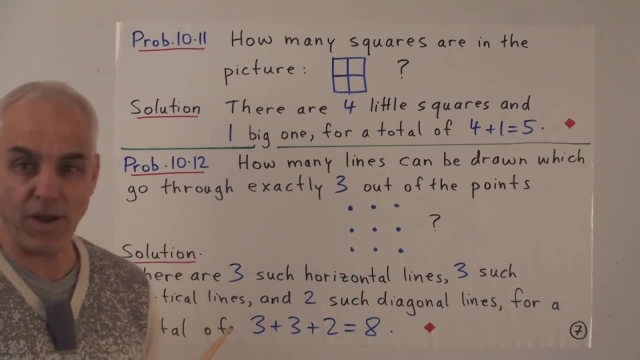 There's another one, There's another one, So there's four little ones, And then a little bit of reflection shows that, well, actually there's the big square itself too. That's also a square. So here's what I would write down. 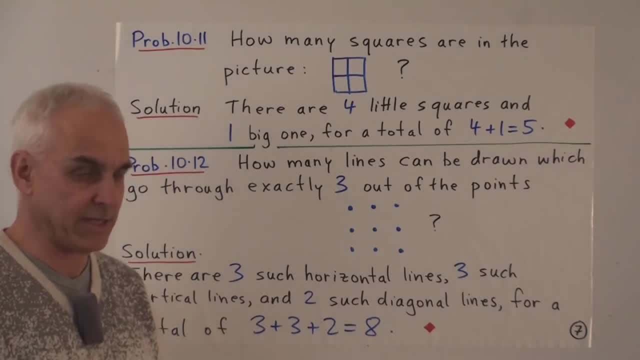 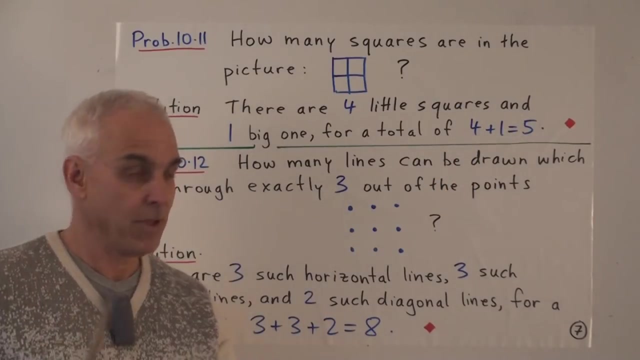 I would explain that So that someone can follow my reasoning. I write down: there are four little squares And one big one For a total of. Now I'm going to do the calculation: Four plus one Equals five. So hopefully someone can read this and follow my train of thought. 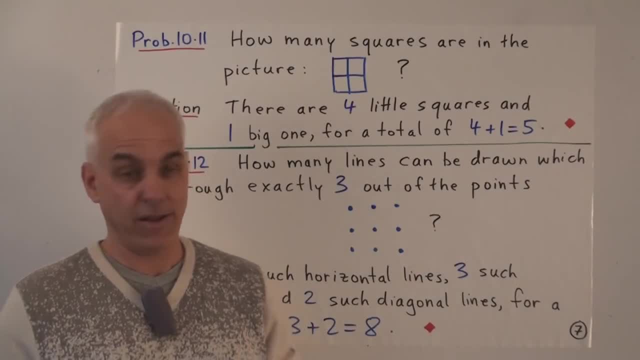 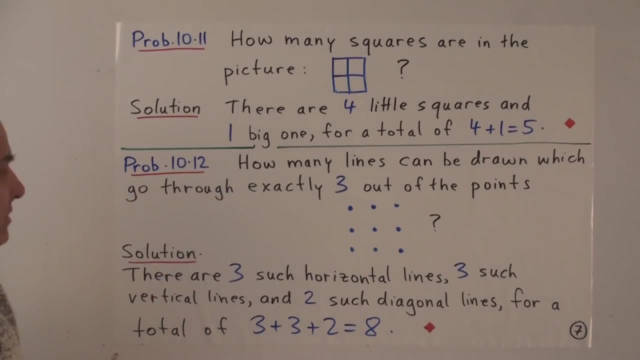 And verify that I've actually made the calculation correctly, That I didn't add four and one and get six. Our last problem: How many lines can be drawn Which go through exactly three out of the points? on this little diagram There are nine points arranged in a square. 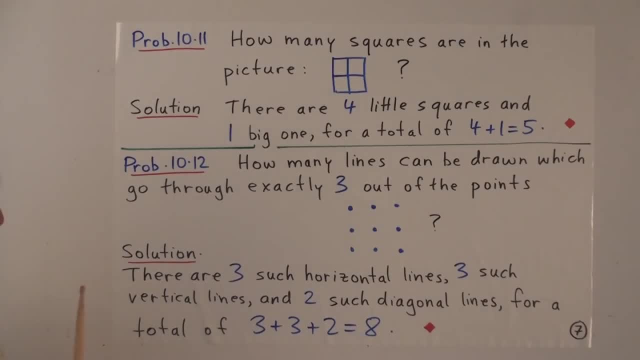 Sort of a bit like this one. And now I'm interested in how many lines can be drawn through exactly three of these points, And by line I mean straight line. Okay, it's a counting question. I want to think about it systematically, So I'm going to try to group the lines into natural families. 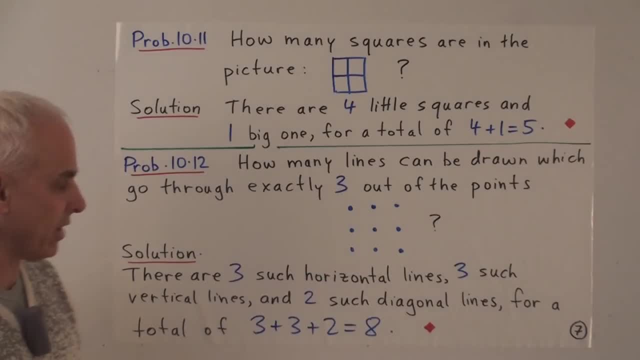 So I'm going to say, first of all, there are three such horizontal lines. There's one horizontal line that goes through three. There's another horizontal line that goes through three, There's another one. So there are three horizontal lines that do the trick. 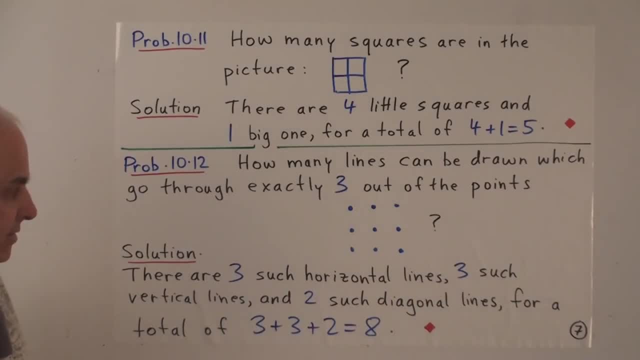 There are also three such vertical lines: That one, That one And that one, And that's not all. Also two such diagonal lines, Because this diagonal line And this diagonal line Can also go through three of the points And I can't see any other lines. 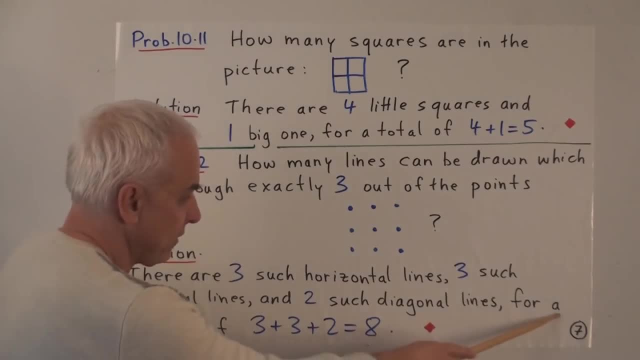 So that's all I've got. So the total is For a total of: And now I have to add this three, This three And this two, And I'm going to write that out as an equation: Three plus three plus two. 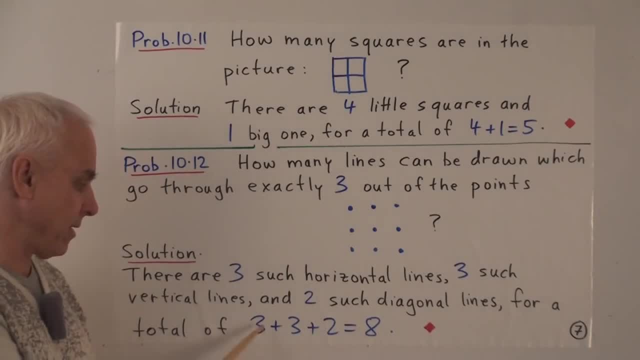 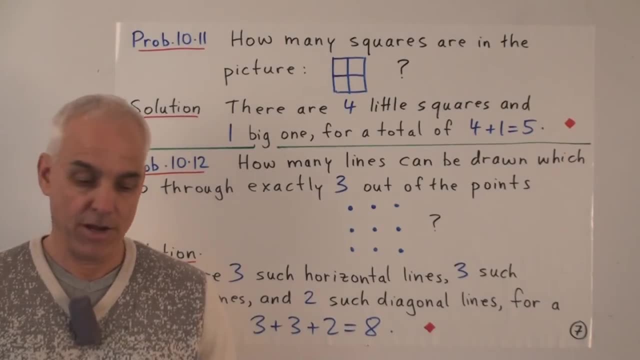 And now I'm going to make the calculation Equals eight. Three plus three is six Plus two is eight, And I'll just write down that: eight. Okay, so that's enough for me. Now it's time for you to have a go. 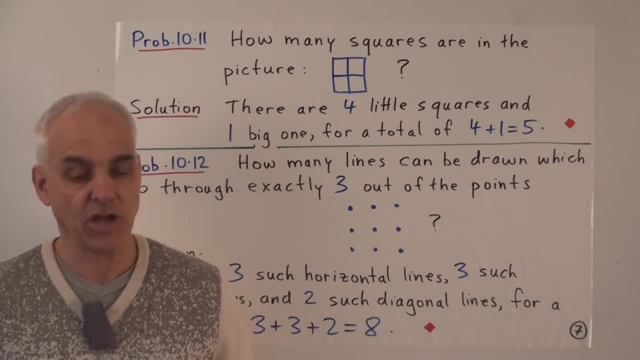 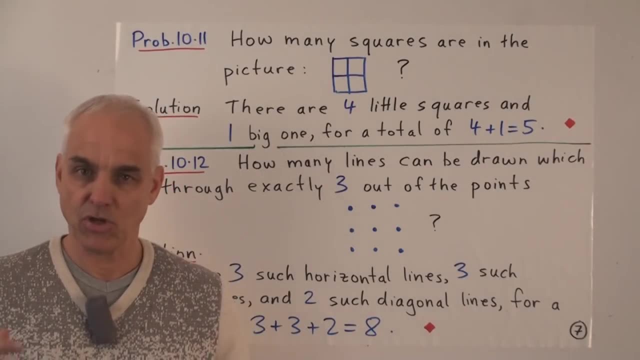 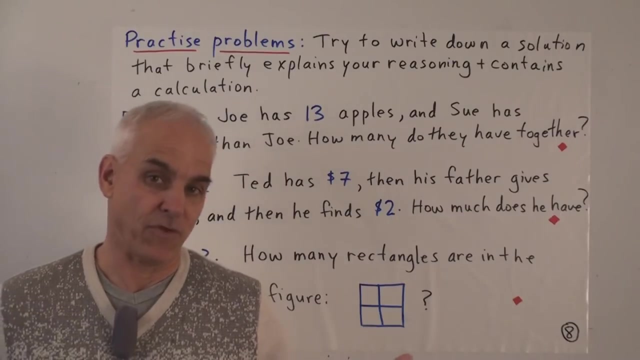 Here are some practice problems for you To practice, not just doing a bit of addition, But also writing out Concise solutions that capture Your trains of thought. So here are some examples for you to practice. Well, first of all, your addition skills. 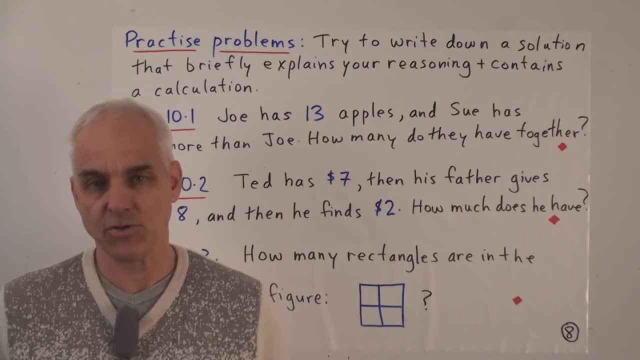 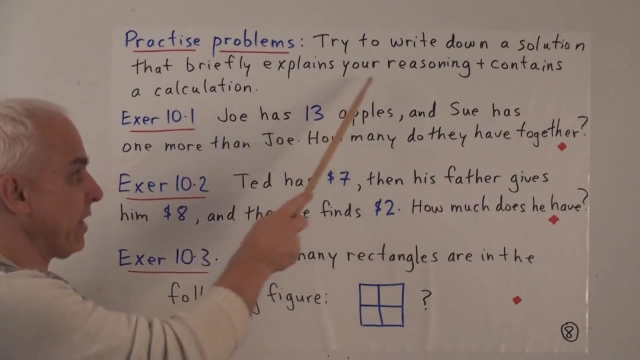 Rather simple ones, But also, more importantly, just to interpret problems And to write out a solution Using words That reflect The problem that you're asked. Okay, we're looking for A solution that Briefly explains your reasoning And contains a calculation. 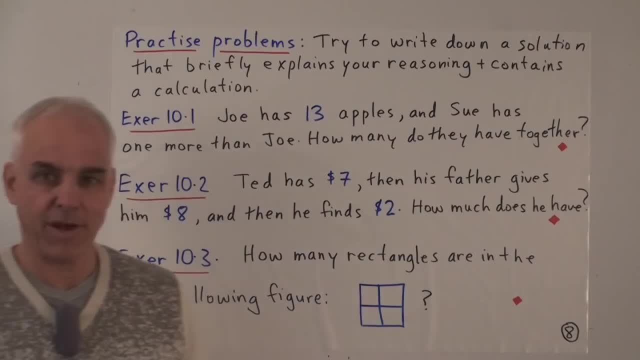 So somewhere in it We would like to have An equation like: three plus four equals seven Or something like that, And preferably Your solution should be a grammatically Correct sentence Beginning with a capital letter, Ending with a capital letter. 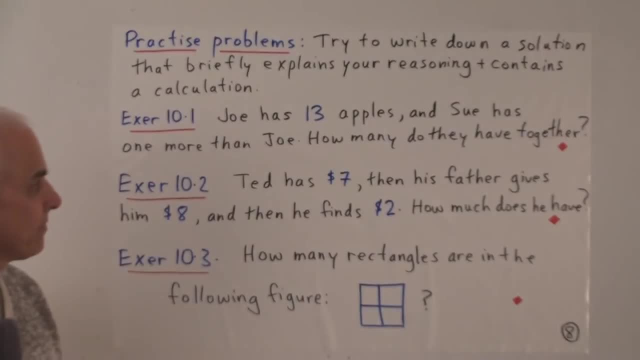 Ending with a period. Reasonable grammar inside First exercise: Joe has thirteen apples And Sue has one more than Joe. How many do they have altogether? Question two: Ted has seven dollars, Then his father gives him eight dollars, Then he finds two dollars. 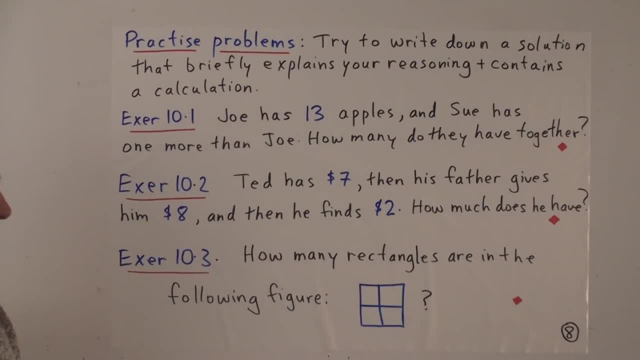 How much does he have? And this third question: How many rectangles are in the following figure? Same figure we've seen before, But now we're counting rectangles, Not just squares. And I remind you that A square like this one here, 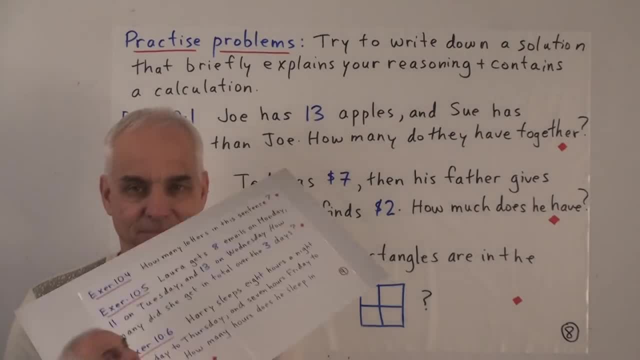 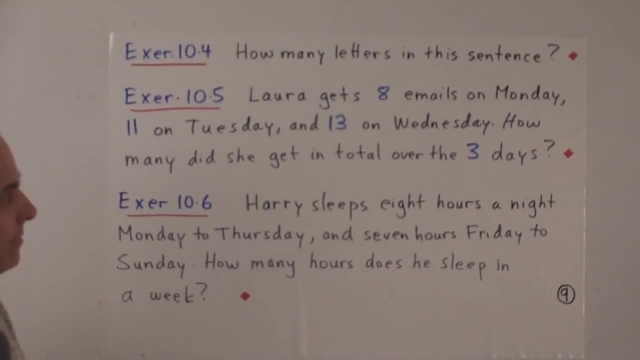 Does also count as a rectangle And in this exercise, How many letters in this sentence? That's maybe not even grammatically correct, is it? But anyway, let's suppose that it is. How many letters in this sentence? It's an addition question. 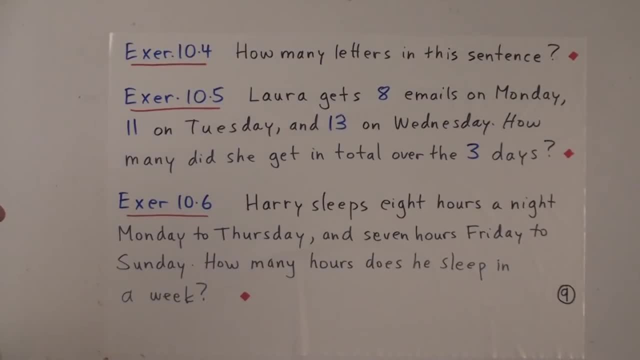 But you have to add up quite a few things. The next one: Laura gets eight emails on Monday, Eleven on Tuesday And thirteen on Wednesday. How many did she get in total over the three days? And finally, Harry sleeps eight hours a night. 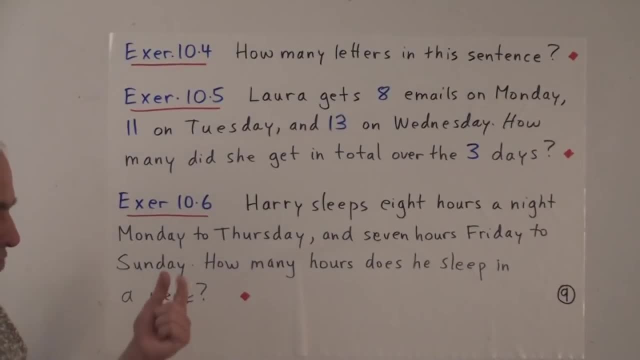 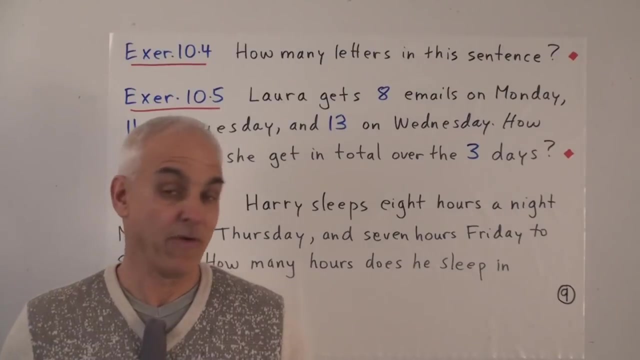 Monday to Thursday. So on Monday, Tuesday, Wednesday, Thursday night He sleeps eight hours And seven hours. Friday to Sunday. Friday, Saturday and Sunday he sleeps seven. How many hours does he sleep in a week? So a chance for you to practice writing down some mathematics. 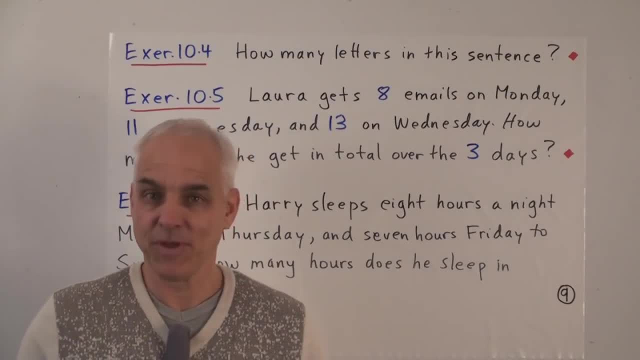 In our next video we're going to go in a slightly different direction. We'll put arithmetic aside for a little while And do some more geometry, But it will be a different kind of geometry, One that you haven't seen before. In fact, it's a geometry that most students don't see very much of. 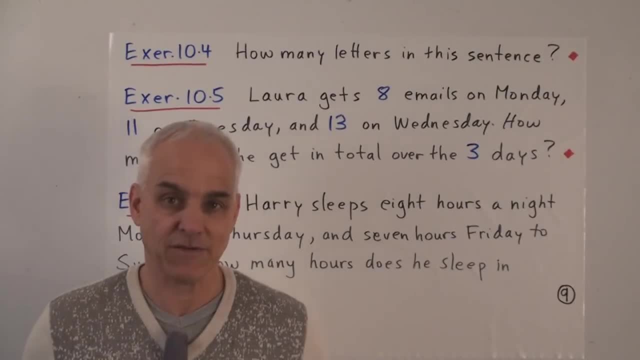 We're going to look at elementary projective geometry, Which is quite a lot of fun and interesting. I hope you'll join me for that. I'm Norman Wildberger. Thanks for listening.